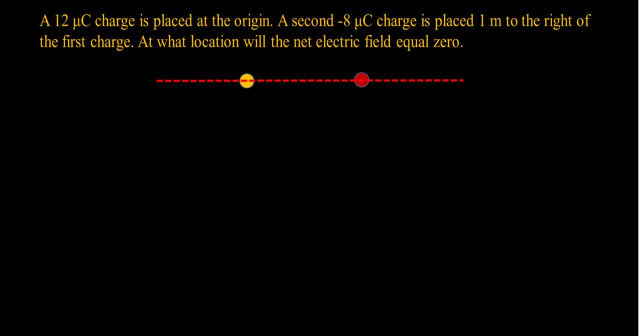 the negative 8 micro column. at which location will the net electric field equal zero? okay, so to handle such a question we need to think about it in a logic based on the definition of the electric field. so I will say I have three different regions. I have region 1. 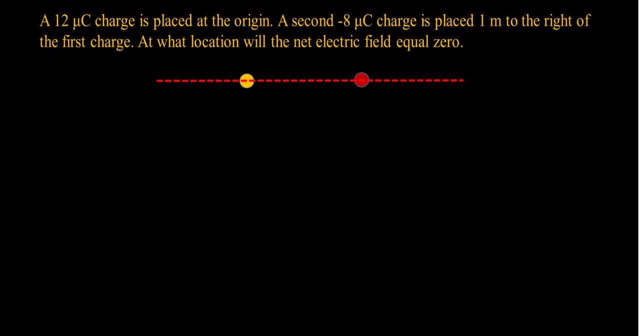 one here to the left of the 12 micro column, the middle between the two charges, and I have region 3, which is to the right, at the right to negative 8 micro column. so I can say this is our 12 micro column. this is here the negative. 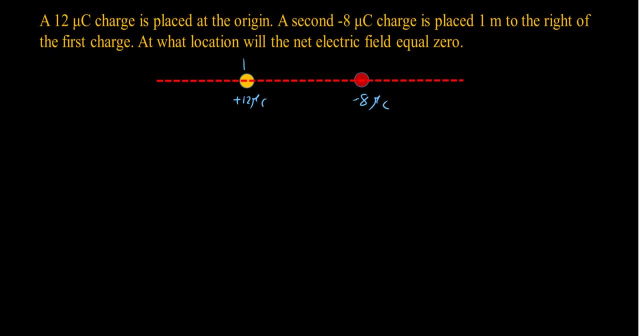 8 micro column. the distance between them is a 1 meter. now the key to figure out where should I start or predict the area where the electric field will be zero between the three regions, is to try identifying the direction of the total electric field in each region. 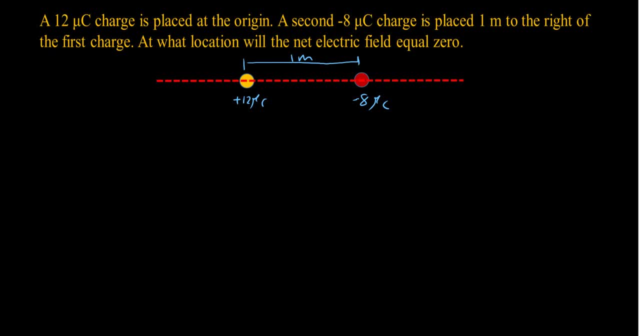 so if I manage to figure out the direction of the electric, the net electric field in each region, I can tell that in this region there is a really good chance for the electric field to be zero. so if I assume this is my point, one in region one which is here as my region one, first of all I will say 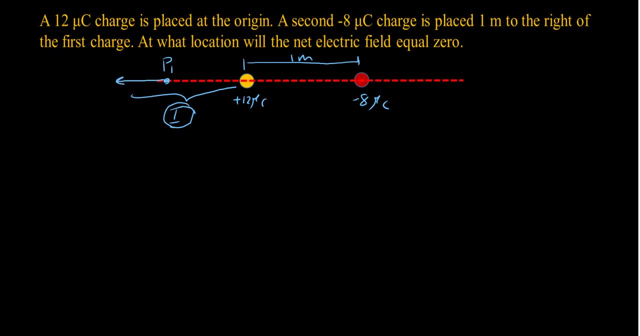 that the electric field will be zero and the electric field will be negative. electric field generated by the 12 micro column will be going to the left, where the electric field generated by the negative 8 micro column will be going to the right. now it might look like it. they are equal in magnitude, opposite in: 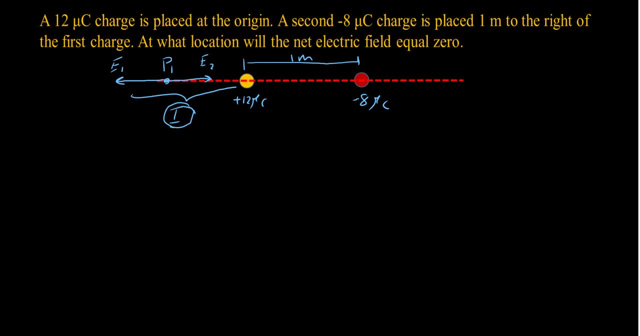 direction. but they're not. because, following the concept that the relationship between the electric field and the distance, it is a squared inverse log and because we are too close in region, one from the 12 micro column. that will make the electric field one always demanding, and it will be. 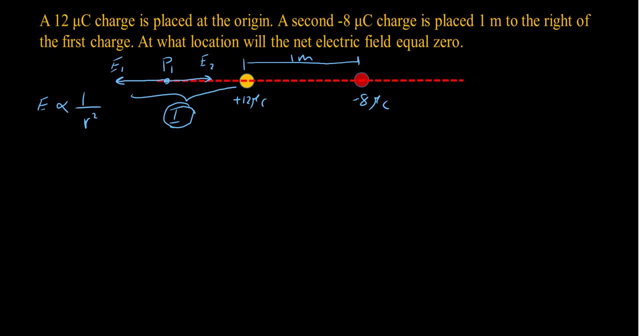 always exist. so the net electric field in region one in one way or another always going to be going kind of like to the left. so region one will be out of the picture because of the 12 micro column. now let's assume in region two I have my discharge. it's somewhere in the middle between the two charges, okay. 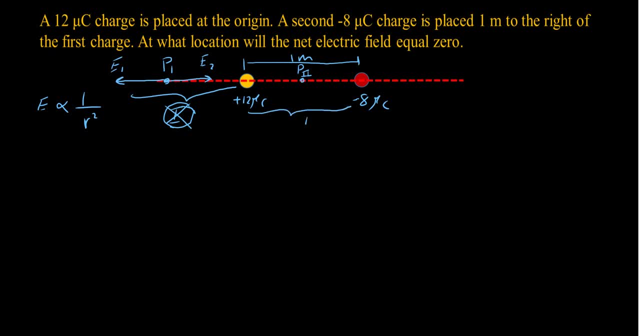 we call it. this is region two. once again, let's identify the direction of electric field one: because of the column, it will be going to the positive x-axis. for the negative, 8 micro column also will be going to the positive of the x-axis and it is very obvious they're adding up to the same direction. 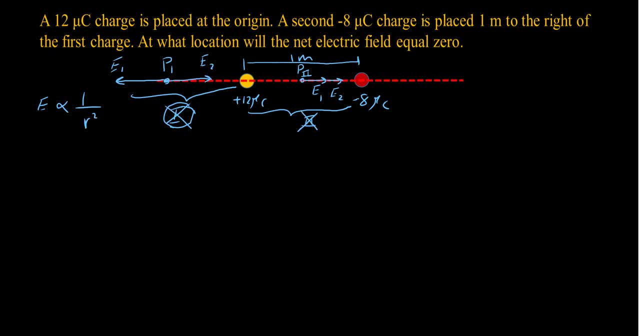 that means there is no way in region 2 to have the electric field to equal zero, because they're always going to be adding up to the same direction will not be ever equal in magnitude, opposite in direction. okay, let's leave us with region 3. so let's see in region 3 how we can handle it. 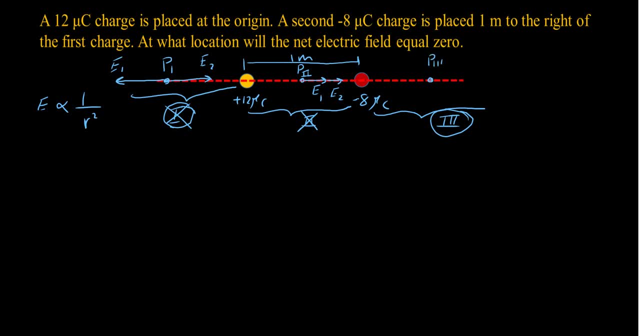 if I put my test charge here, so it's p3 or region 3, the electric field generated because of the 12 micro column will be going away from it, that's e1, where the one generated because of the negative 8 micro column will be going. 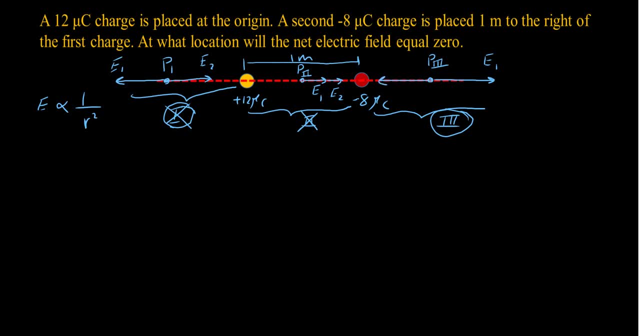 you toward the negative 8 micro column. now, looking at this will give us a really, really good chance of having a point in region 3 where the electric field of e1 and e2- they're going to be equal in magnitude, opposite in direction, and that will give us a good chance that at this position 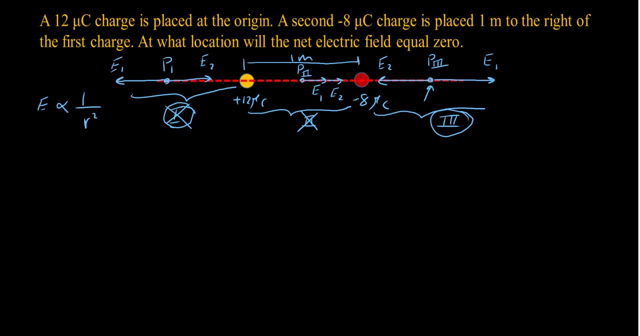 there is a chance to have the electric field total equal 0. okay, so based on this, we need to start doing our calculation around region 3 and follow the formula. so what i'll do? i will erase all these descriptions here and start identifying the distance and few items. that's again our positive: 12 micro column. negative: 8 micro column. 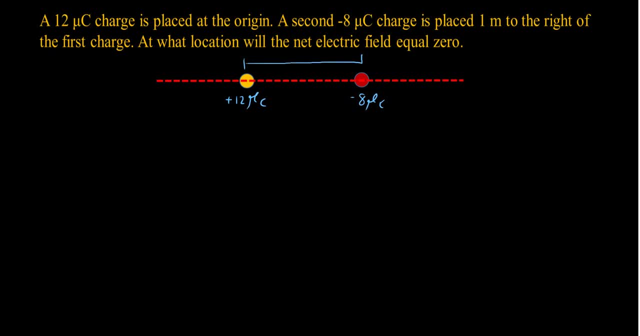 the distance will be 1 meter. and we said, somewhere at region 3, I will have my discharge and the distance will be, let's name it as X. okay, now we said the electric field of e1 will be this way: electric field generated because of the 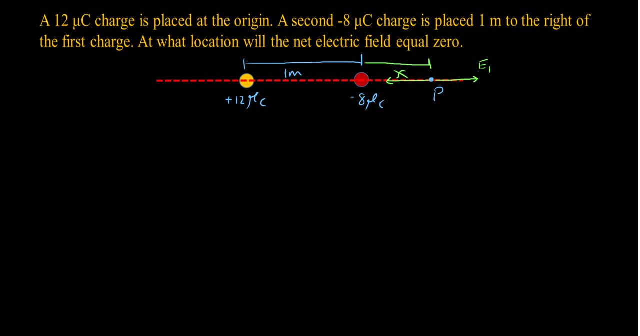 second charge, the negative 8 micro column will be this way, and we said here at this point: P, the total electric field will be zero, which mean e1 is going to equal e2. so okay, Q 1 divided on our 1 square, which is the distance between the 12 micro. 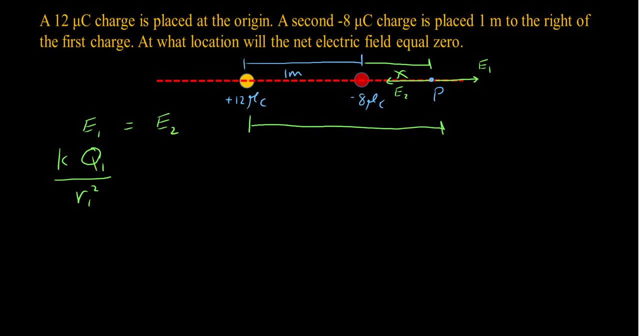 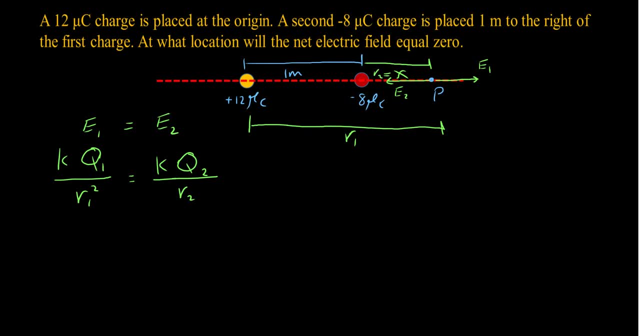 P, so it is X. that's what we are too. all right, let's replace the values. that's kq 1 over 1 plus X all square equal K Q 2 over X square. we can eliminate the constant K. we can continue calculation a bit here. all right, now I can place the values now. 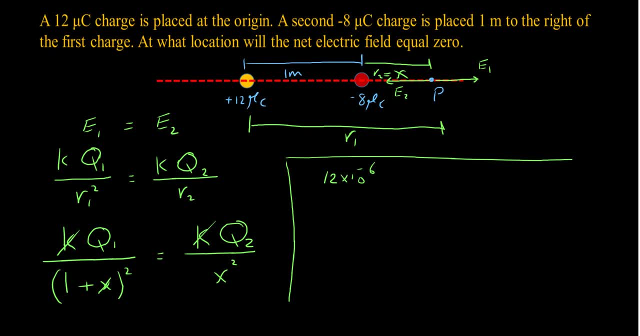 it's a 12: 10 to the power minus 6 over 1 plus X, 8, 10 to the power minus 6. it's all X square. you can take the micros off to cross multiplication. that will give us 12 X square equal 8. 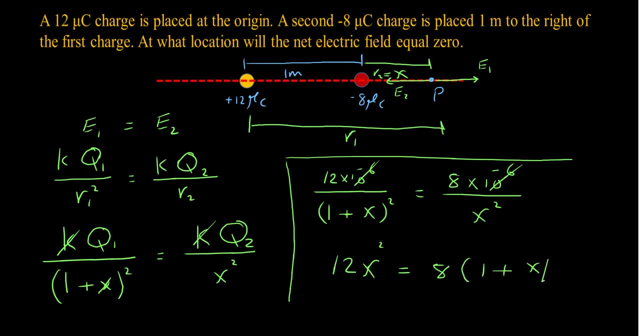 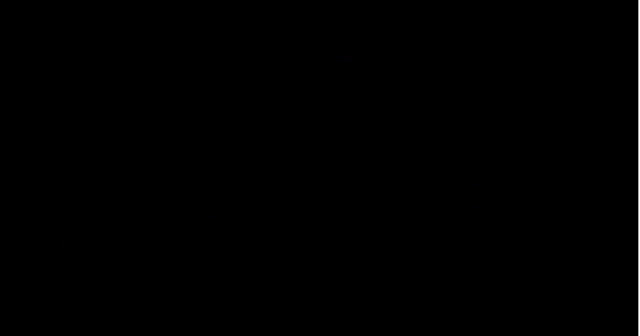 1 plus X. all right, square. all right now, what I'll do? I will take the square root for the two sides and that should give me that won't give me. if I do the square root for 12 and also for 8, that will give me this. 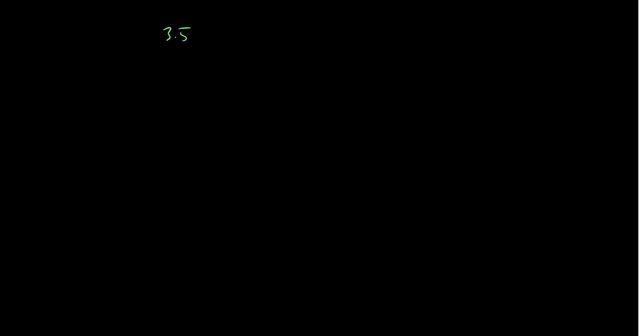 3.5 X, because X square will be X on the square root 2.8, and 1 plus X. can expand our form, rearrange it: 3.5 minus 2.8, X equal 2.8 and X will be 2.8 divided on 0.7. doing that, it's gonna give me 4 meter.